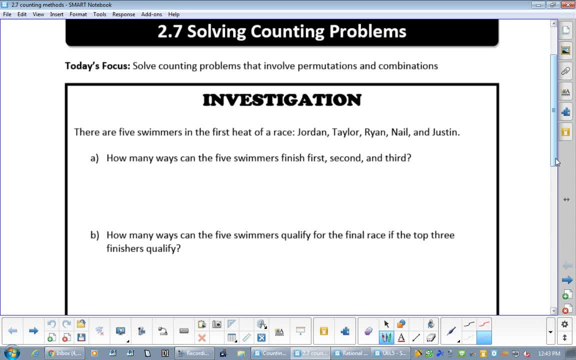 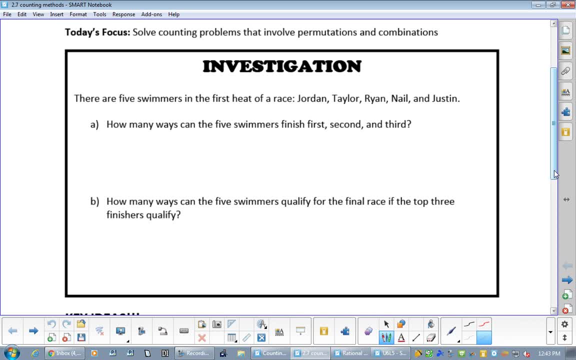 foundational stuff. Now, if you look at this investigation very much like the quiz, do you see how A is very different than B? Okay, what is A specifically talking about? What are they trying to grasp at? Okay, sorry, Okay, A would be what Perm? or a com? Okay, are there specific positions? Okay, so first, 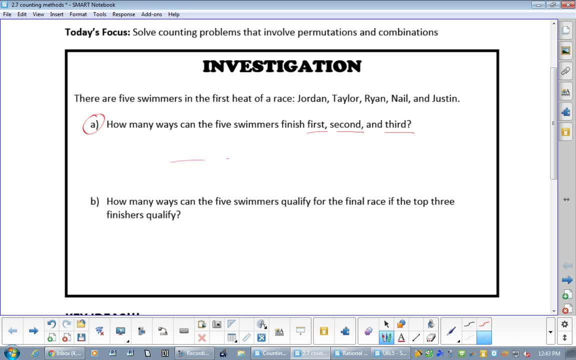 second and third. So when you see that you're going to write down first, second and third, Now how many ways can you get first? We have five people. So five people can get first, then four and then three Or five. 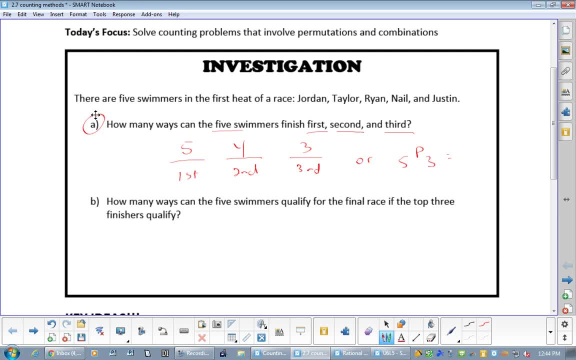 pick three. So there's 60 different ways. So when you see these positions, order matters And if you're like: well, I don't see how order matters, just ask: Well, is it different than getting first and second? 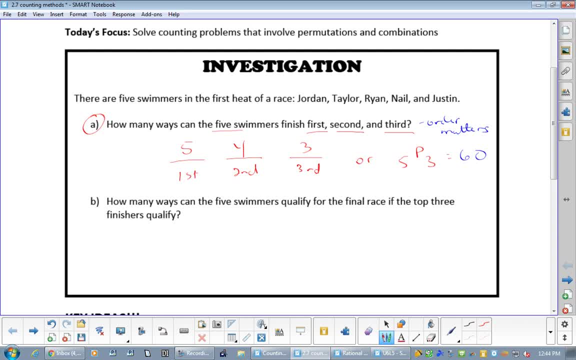 Ask any Olympic athlete, right, What's his goal? same thing as silver, right, And this- and this is this- is the absolute truth. If you win silver in hockey in Canada, okay, and I've heard this right from the actual- uh, like I got to see, I got to talk to Hailey- 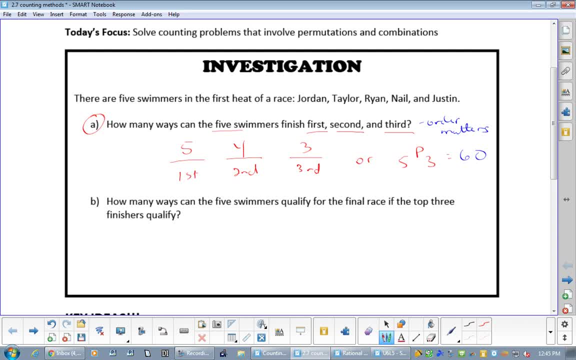 Wick anesthesia week after they won the gold medal last Olympics. who's that? she's captain of the women's uh hockey team. yeah, and the year? no, two years was it? yeah, the Olympics before they won silver, and she said that that's something you just put in a drawer and you forget about. 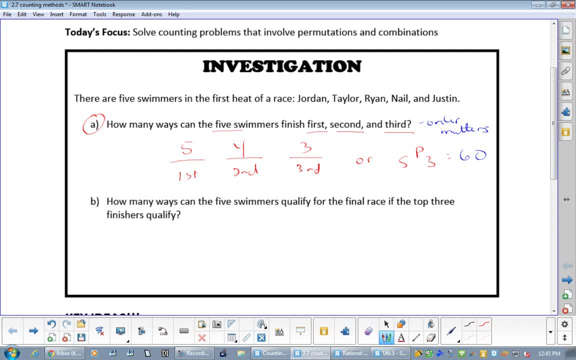 winning silver in hockey for Canada. is not that that's a disgrace for them? it really truly is. I'm not saying that as a fan for them. it's a disgrace, right as a uh, the US and Canada. whoever gets gold, that's the winner, and whoever doesn't get gold is a loser. that's just what it. 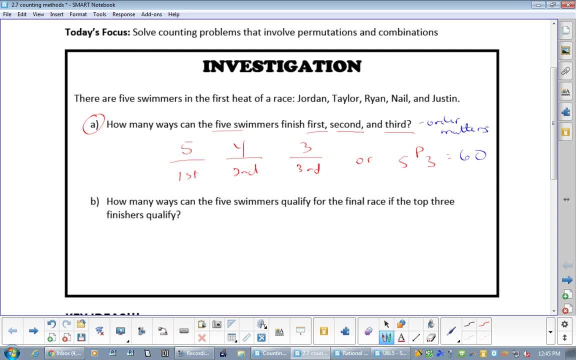 that's how they, that's the truth, right. that's right from their lips, not me going: oh yeah, if you don't get gold, it's nothing. so I think they would argue that gold and silver are very, very different. right, Getting that is. getting a gold is very different than a bronze or a. 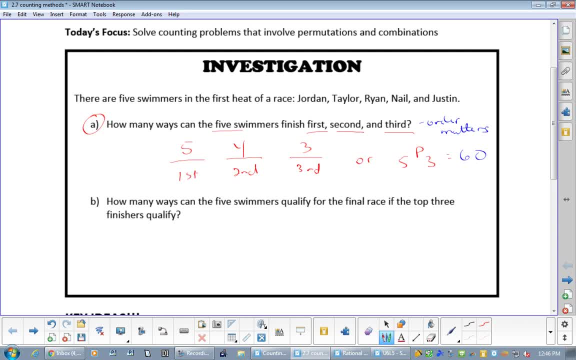 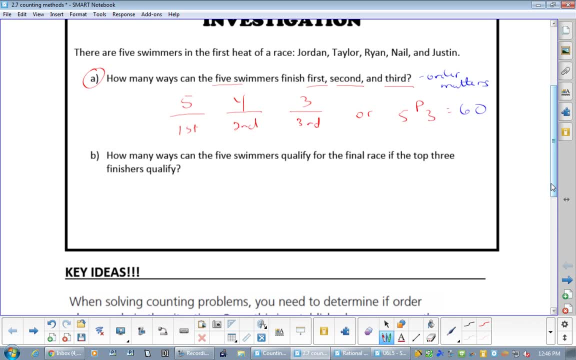 now I could be honest. if I won a silver medal in the Olympics, I wouldn't be putting it in a drawer. okay, I'd probably be wearing it every day. Now, how many ways can five swimmers qualify for a final race? 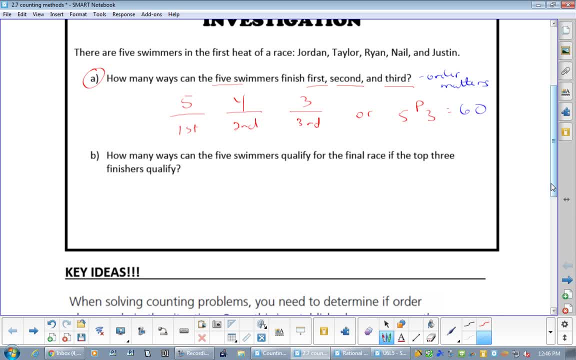 if the top three finishers qualify, That's see, it doesn't matter if you came in third, So you get to go on, right, That's all that matters. I get to go on And, yeah, you can like. if someone said to me: like if I came in third. 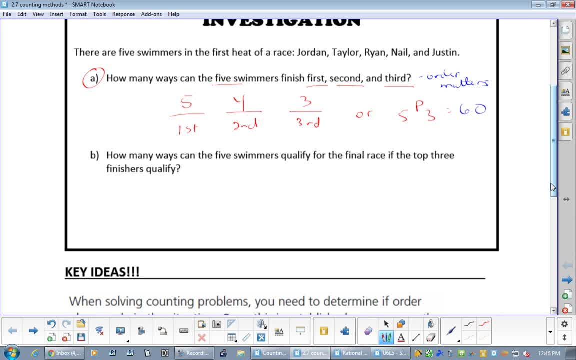 and they're like: yeah, you came in third. I'm like you know what, It doesn't matter, I'm going on right. So that is five, choose three. Also can be written like this: right Now, this does anybody remember? I want to see if anybody remembers. 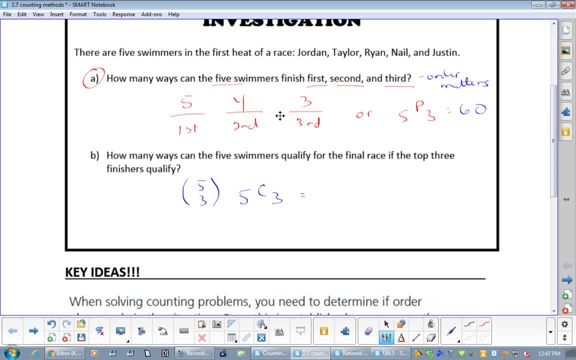 I'll be impressed what this is called When I do like this, this, this, When you draw three lines and you go five times, four times, this actually has a name Something: counting principle, Fundamental counting principle. That is the same thing as a permutation. 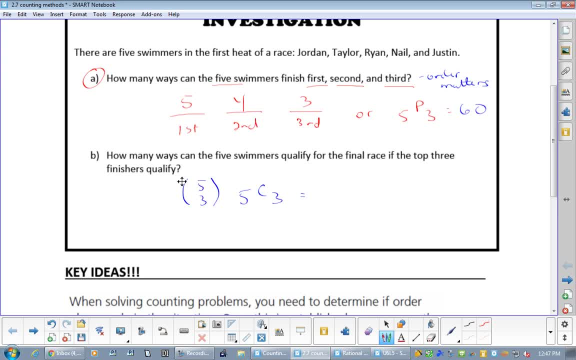 You can't use the fundamental counting principle for comms. okay, This is the way you're going to do it. So you get five, see three, and you get ten. And yes, you will always get a smaller number for combinations because 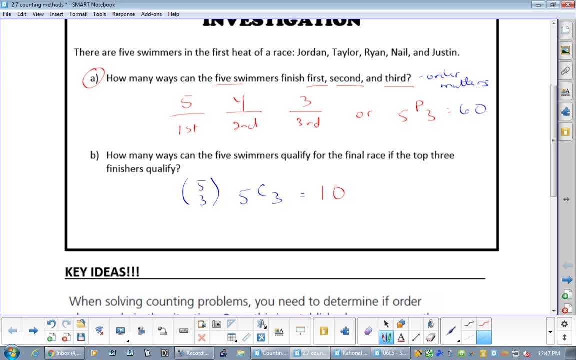 you know what order doesn't matter: First, second, third, that's the same thing as third, like third, two, one. I don't care what order. Who's the top three, Like, I'm the top three. 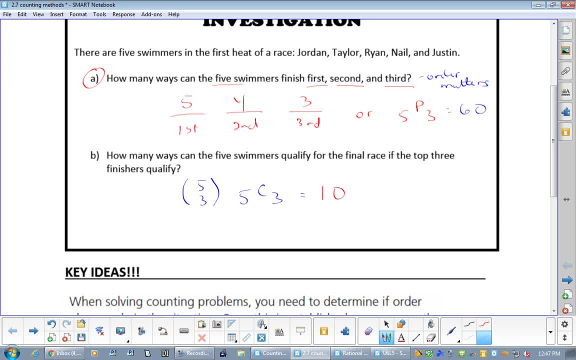 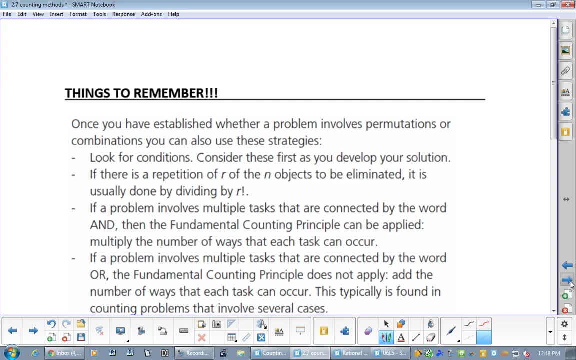 Okay, over here, Right, And you? you know those people can sit there and talk about: oh, I came, I came in before you. I don't really care, I'm going on. Okay, Now we talked about. if there's things to remember, look for conditions. 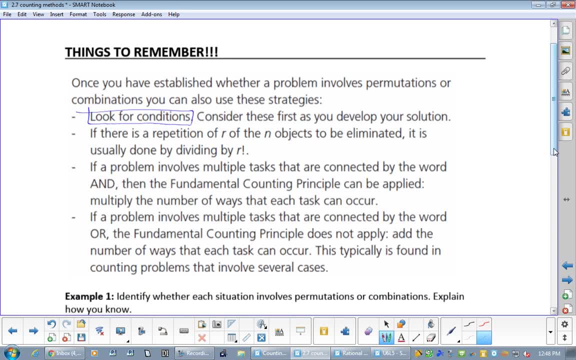 Okay, That's huge. We'll talk about that more today. The second thing: if you have a repetition of r, objects, divide by r- factorial right. We did that on yesterday's quiz. If a problem involves multiple tasks that are connected by the word and the fundamental counting. 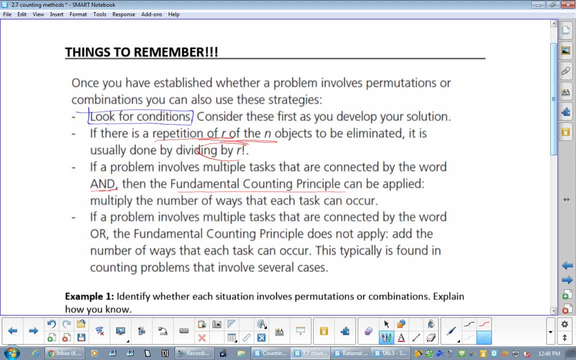 principle can be applied, and a multiple and and you multiply. okay, So you just multiply the number of ways each task to occur. Now, and we talked about this a bit yesterday- If a problem involves multiple tasks that are connected by the word, or we want to, 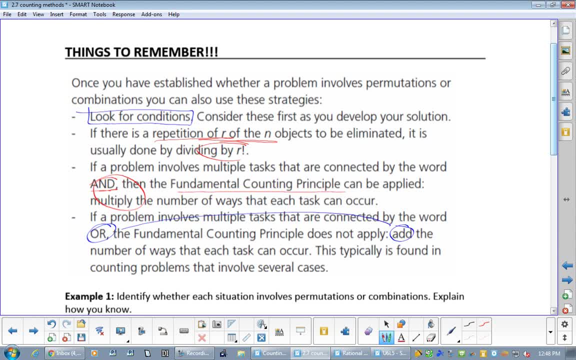 add. okay, we want to add the number of ways. So you really want to be like, of course. I want you on my test and I want you at the diploma. I want you circling ors, I want you circling ands, because I need you. 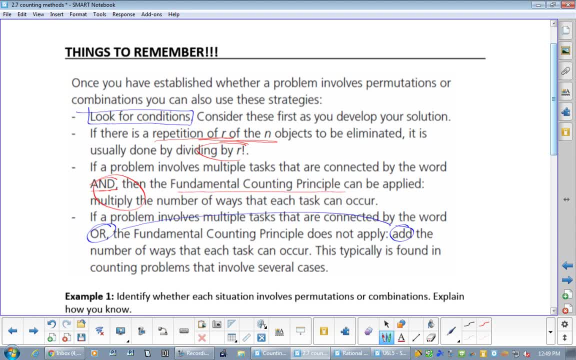 to have a definite plan when you do these- And I was even talking about another with another math teacher, because for 99% of math teachers, this is the most difficult of all to even teach. And If, if anything will help you the most on that diploma, it's you going and writing this test. 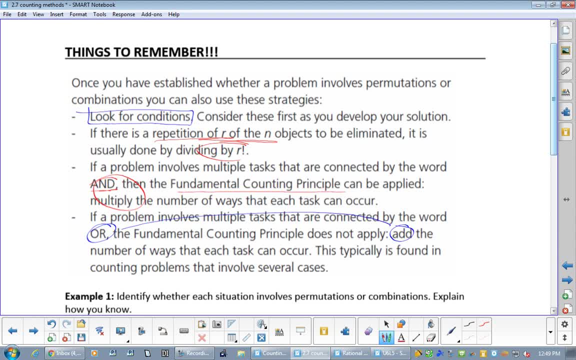 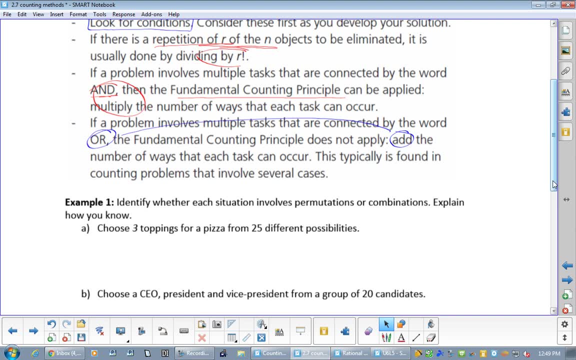 when you're really well rested and you're thinking clear. okay, So that's why you're not cramming for this test. The night, the night before this test, should be your most relaxed. okay, You might be able to be reading a few study sheets over every so often, or whatever, but 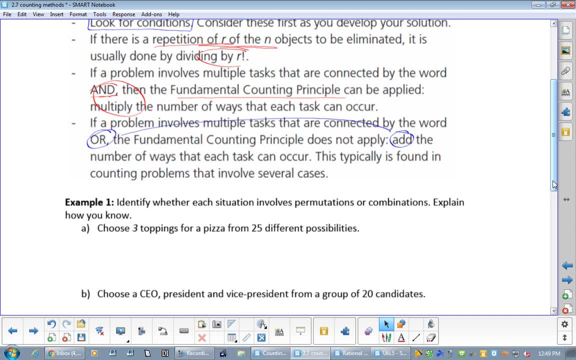 you know, you got to be on your game and this is the biggest. last unit, this one and the next one are the three units that you really got to be thinking: whoa? okay, so okay, we got an, and here order matters okay. 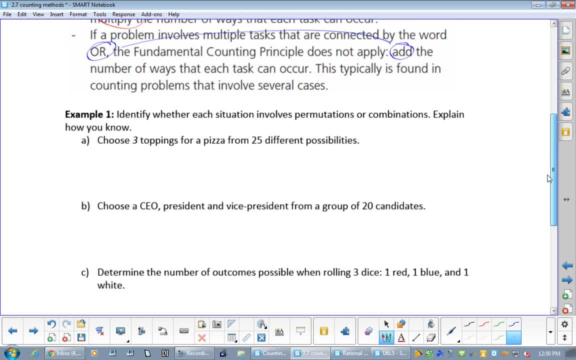 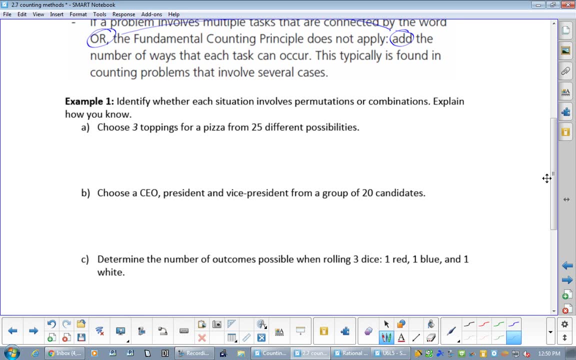 and then there's an or scenario. Okay, I know what to do now, So let's just look through these and just see how we would. we would do these, okay, Now? choose three toppings for a pizza from 25 different possibilities. 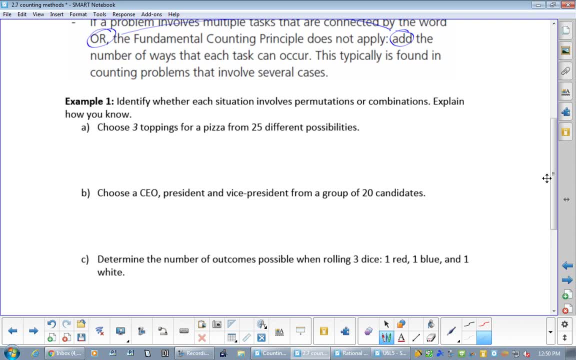 Now the question: is it a perm or is it a com? and they may be that simple A question, a multiple choice question, could be: which of the following is a permutation? And they'll give three scenarios and you got to pick the one. okay, 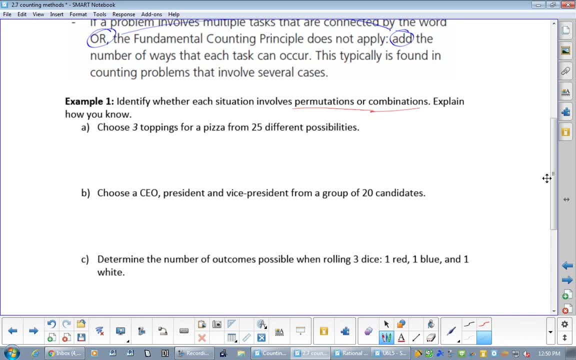 So when I'm reading over that diploma while you're doing it in the gym- because that's the only time I'm allowed to do- it- is the exact time you're doing it. I do not get to see it a minute before and I only get it. 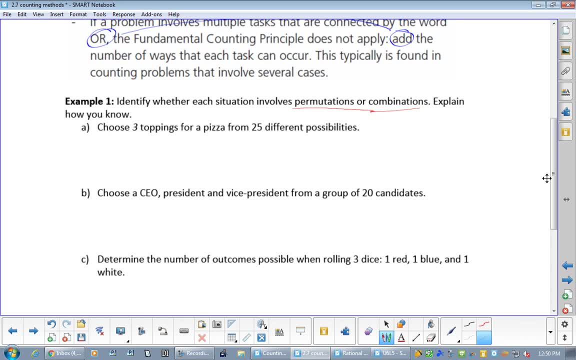 until you guys are out of there, right? So I'm looking through these and I'm like, okay, they better be getting this one. okay, I hope they knew this one. So how are we going to know, by looking at A, if it should be a perm or a com? 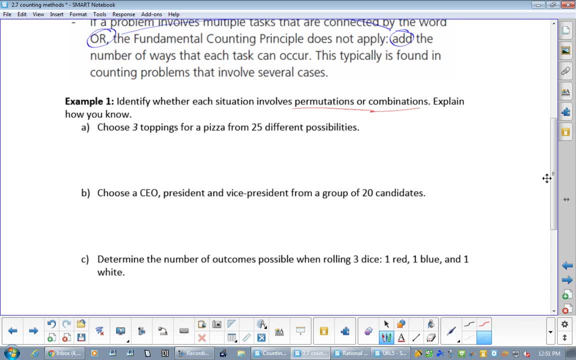 It will not say that. sometimes, though, It will not come right out and say: order matters or order doesn't matter. Yes, Okay, awesome, You can't have cheese, cheese, cheese. That's the first thing, and that will help you with both of these, right. 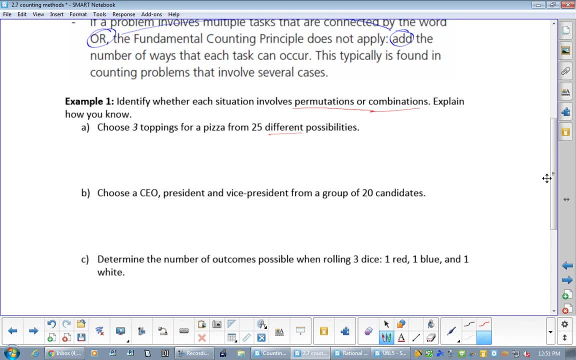 So repetitions are not in there, okay, So you don't have to divide by repetitions. Now I want you to think about When you choose three toppings and you order. have you ever been conscious about making sure you ask them in the right order? 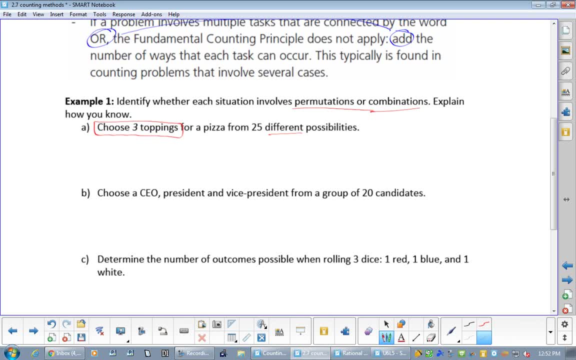 No, okay, They will do it the way they're going to do it. So when you're just choosing three toppings, that order shouldn't matter, okay. So then you would go 25C3, okay, If you have an argument. 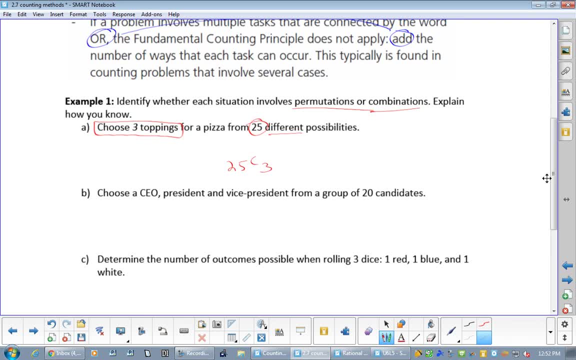 I'm going to go 25C3.. I'm happy to hear it. No, I mean, yeah, I just realized 25 choose 3, not 25 choose 3.. Right, And we're going to say order does not matter. 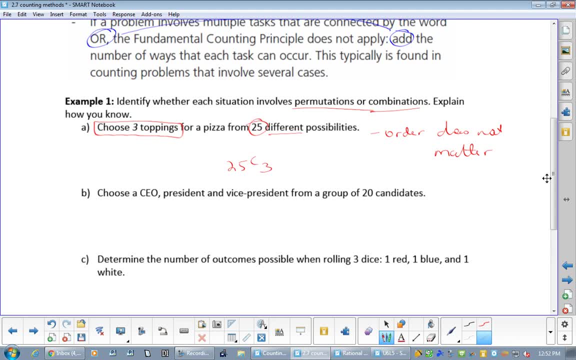 Okay, now some of these. right from the beginning you're like, oh okay, that makes sense. Now, I might not have got that if it was a test. Well, the whole trick is doing. enough of these. so then you kind of 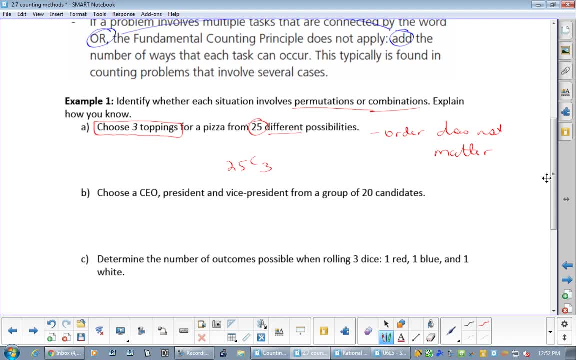 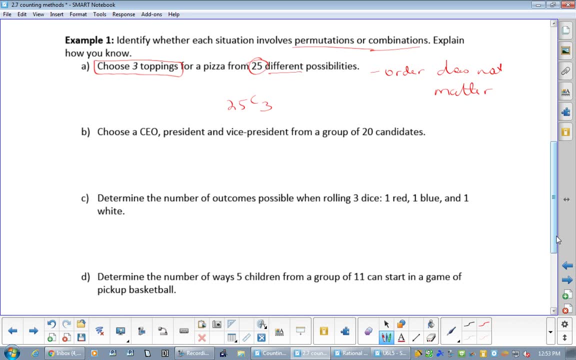 Well, remember, oh yeah, I remember doing this one in class, And if you can remember doing it in class then you're going to have a better chance of it. Okay, B, perm or com, and why? Okay? Okay, I've heard com and perm. 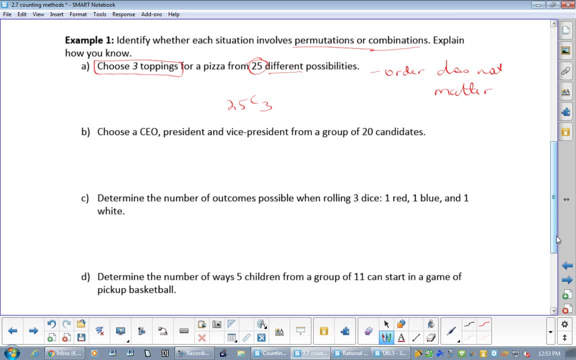 You're saying com. Okay, your reasoning for com. It doesn't say they have to be picked in a specific order. It's assuming that these are all different, right? Yes, Yeah, if I got, chose to be president or chose to be CEO. those are different. 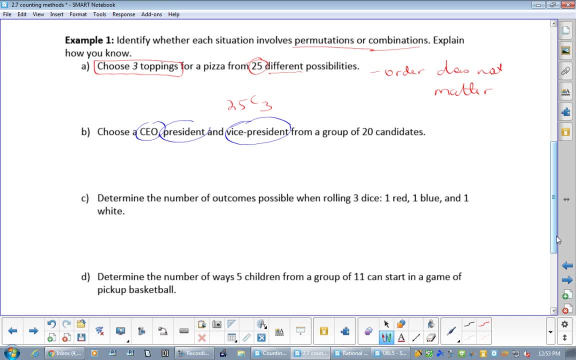 Right, Those are highly unique, right? Okay? So we're seeing specific, Specific positions, Order matters, okay. So when you see specific, defined positions, order matters, we're going to go 20P3.. Okay, Okay, determine the number of outcomes when rolling. 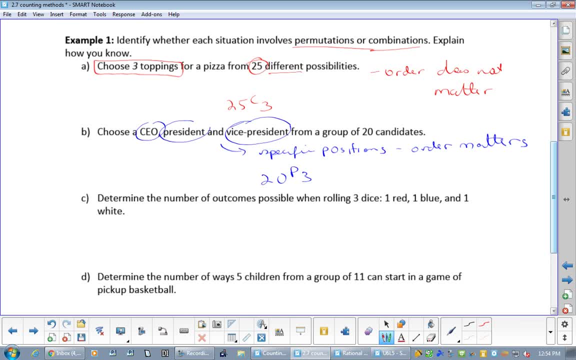 Three dice: one red, one blue and one white. We're going to assume six, okay, But they will be very good at that. So we would say six-sided okay, And if this was a diploma question, it would definitely say six-sided. 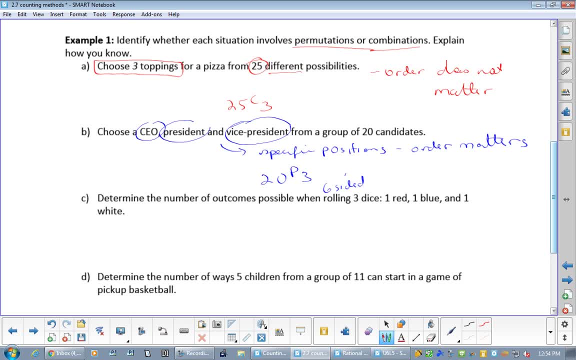 So the number of outcomes possible when we got three six-sided dice, one red, one blue and one white. Do we have a pass option? Perm or a calm? Do we have a pass option? Yes? Okay, It's a green card. 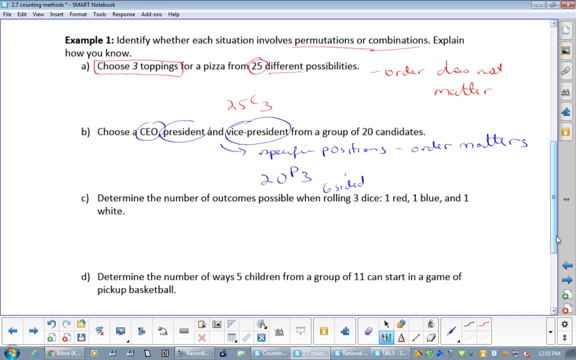 Green card. Yeah, Can I just say you're getting a green card. Yes, I can show you what that gives. What do you want? Okay, Do I get a big? Yes, big when it comes to and policies. Okay. 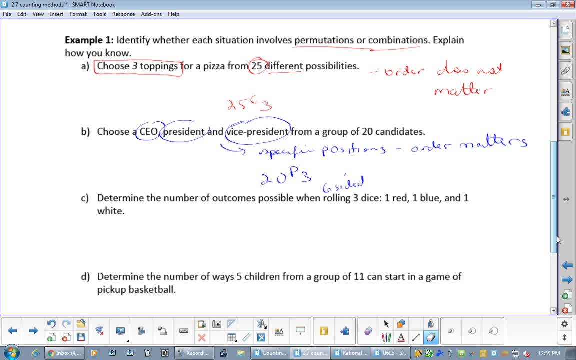 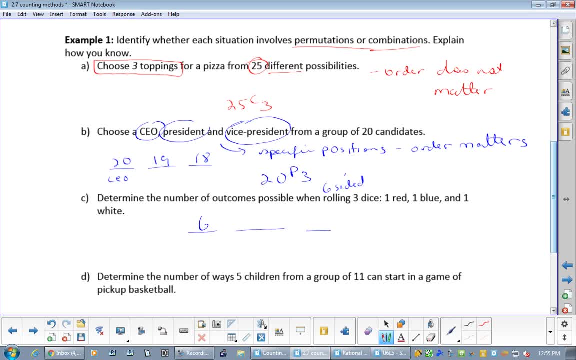 the first dice: how many choices are there? the second one: do you see how this is not really a perm or a calm 8? now, this is called fundamental counting principle. but so I don't want you to think that fundamental counting principle always means perm. if you count down, it will be a perm. so if you use 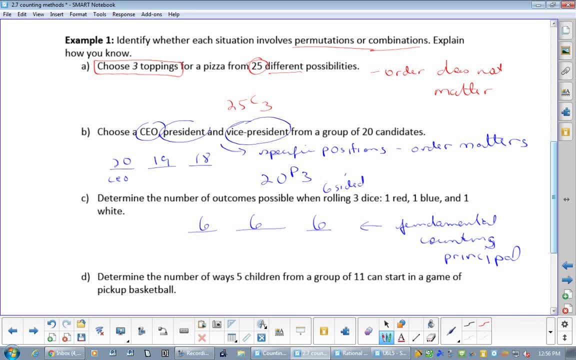 fundamentals going 7,, 6,, 5,. that's a permutation, But if you're going 7,, 7,, 7, right, that would be just fundamental counting principle. Okay, So sometimes, because this is fundamental counting principle as well, 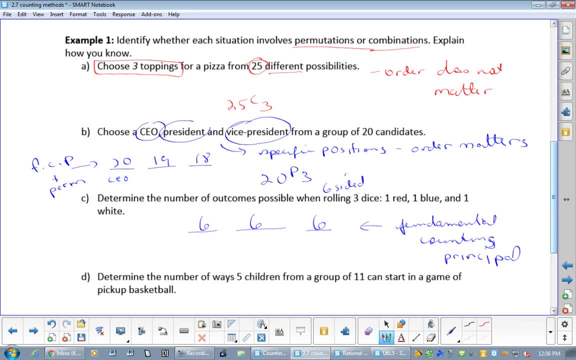 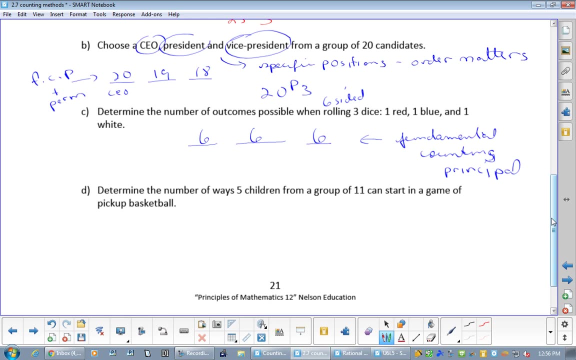 plus a perm To be both you need to be counting down. Next one Determine the number of ways 5 children from a group of 11 can start in a game of pickup basketball Combination. Yeah, so order doesn't matter. 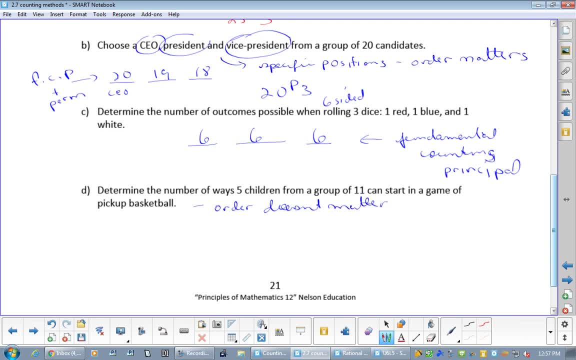 So how would you solve this? 11, C, 5.. Now, if there was specific positions, then it would be 11, pick 5.. Does that make sense? Okay, so if you, just because when you play pickup basketball. 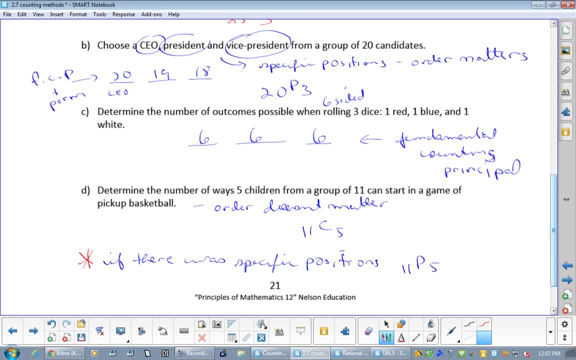 it's always lame when someone says I'm going to be point guard And you're like: okay, man, like we're just playing basketball here, I don't know if you need to right. So that's implying the pickup is applying that oops, order doesn't matter. 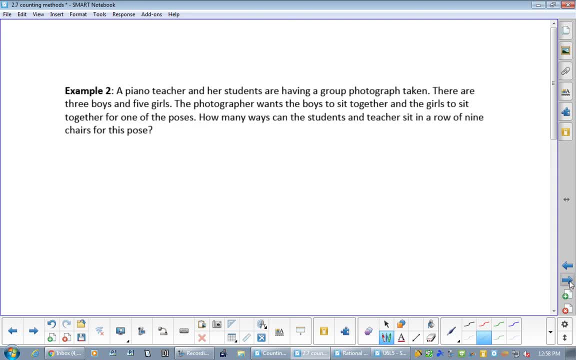 What am I doing here? Okay, So now this is a huge one. okay, Now I'm going to show you a way to do these. There's a lot of different ways, And I've been doing these long enough that I have found the one. 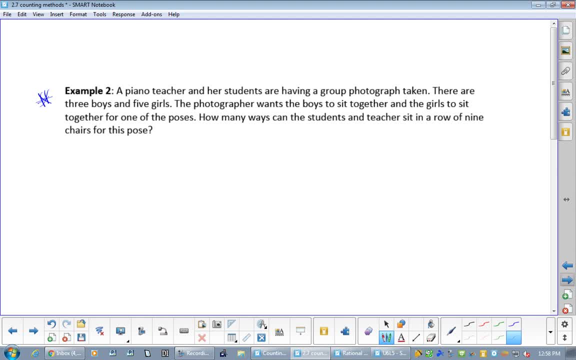 that students seem to really understand. So if you think this one's complicated, there's way more complicated ways to do these. But I want you to kind of listen to the scenario first, because it's a complicated scenario. A piano teacher and her students are having a group photograph taken. 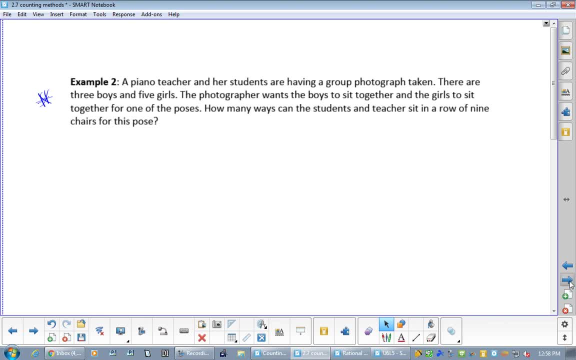 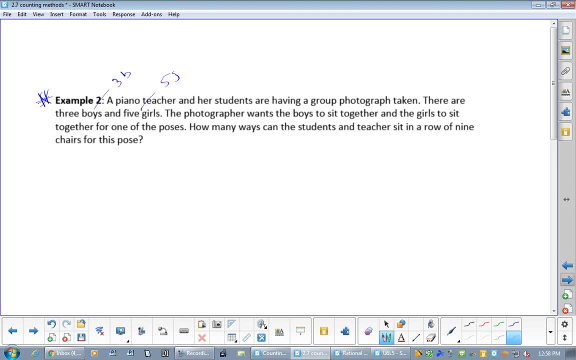 There are three boys, So we have. oh, why is this pen not working? I have three boys and I have five girls. The photographer wants the boys to sit together and the girls to sit together for one of the poses. How many ways can students and teachers sit in a row of nine chairs? 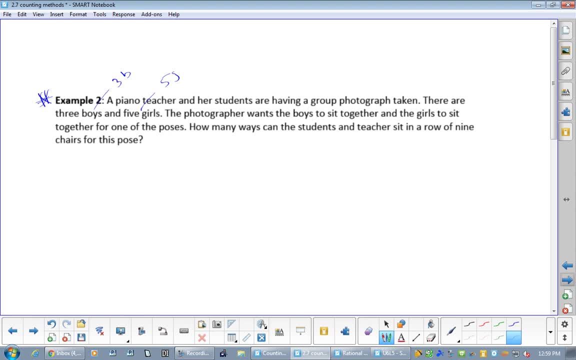 Okay, So we have three boys. We have three girls chairs for this polls k, so this one isn't as clear-cut as uh. so we have three boys, five girls and one teacher. uh, no, this is how you have: girl, girl, girl, five girls. 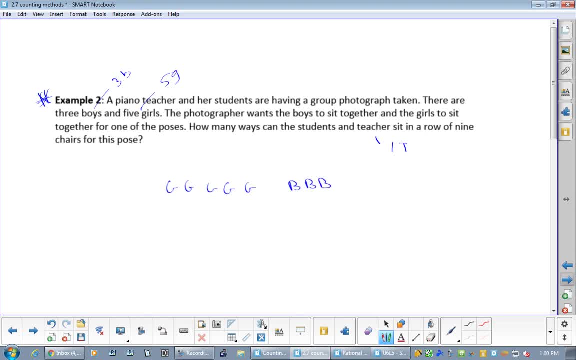 you have three boys and you have a teacher. now let me help you understand what's going on here now. first of all, the girls must stay together, but they can switch around within here. these boys must stay together. hold on, these boys must stay together, but they can go. 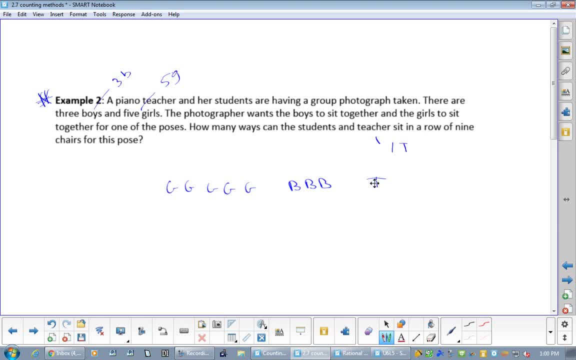 and switch their orders within here. the teacher just once. obviously not going to happen there. but not only that. we could have the three boys first, then the five girls, then the teacher. we'd have the teacher, the five girls, the three boys, we'd have the teacher in the middle. we haven't even done that. 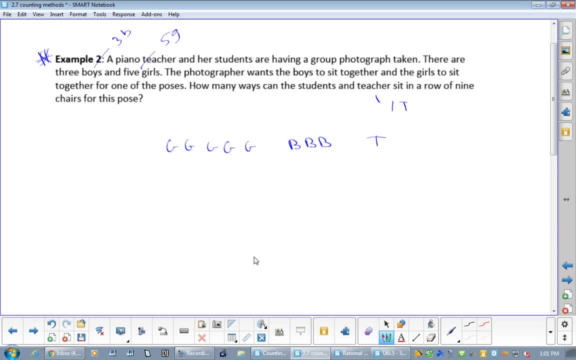 we haven't even done that. so first of all i put boxes around because these have to stay together. those are like three different things now: three entities, there's three groups. how many ways can you change three groups? six ways, three factorial, so just to move the three groups. because 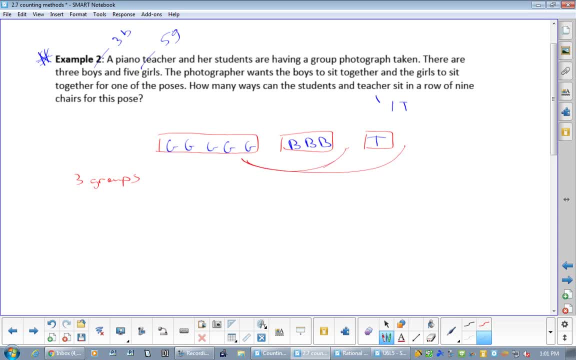 this can go here and here. right, this can go there and there. so just the three groups. just to arrange them would be three factorial. does that make sense for the three groups? how you could be then do within each group how many ways- so i go times- how many ways can you mess with that group? 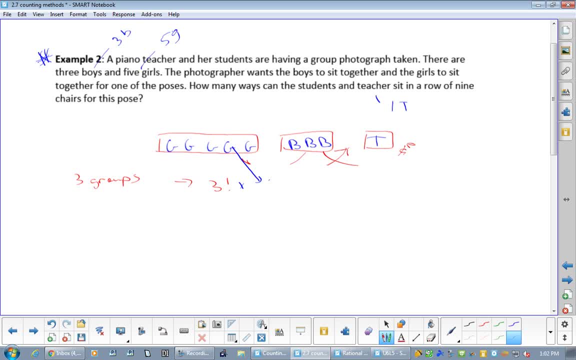 just in the group. how many ways can you mess it? five factorial in this group, three factorial and in this group would be one factorial. i'm just putting that to be consistent. so its number of groups, and then within each group, and then within each group, and as we, as we go along in the unit, you'll see we'll have other ones where. 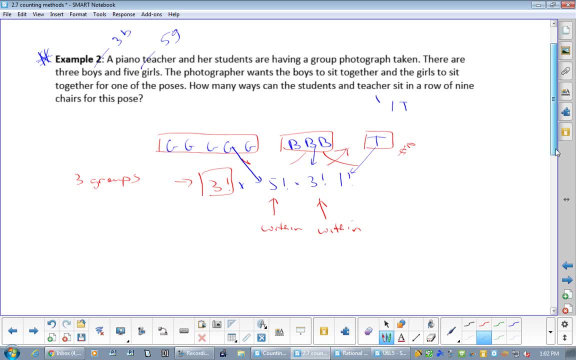 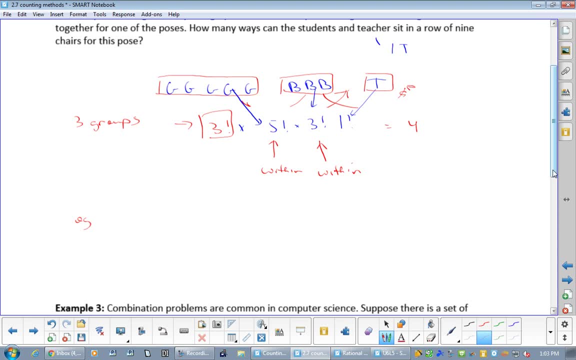 maybe it'll just be one group, ok. so an example like this, or say: anyway, if you multiply this all together, you get four thousand three hundred twenty. but if you had four boys and seven adults, how many ways could you arrange if the, the, the, the, the four boys must be together? 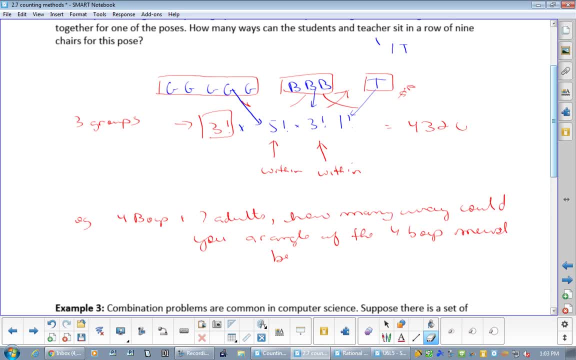 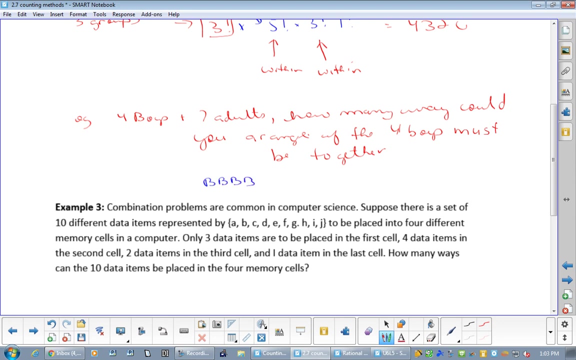 this is more common if the boys, for boys, must be together. so you have the four boys. get 10 really going to be listening this because you're just distracting people, that, they're distracting me. so you have the four boys, and then you have the one, two, three, four. 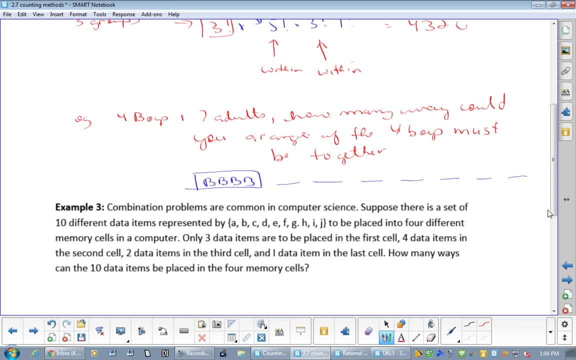 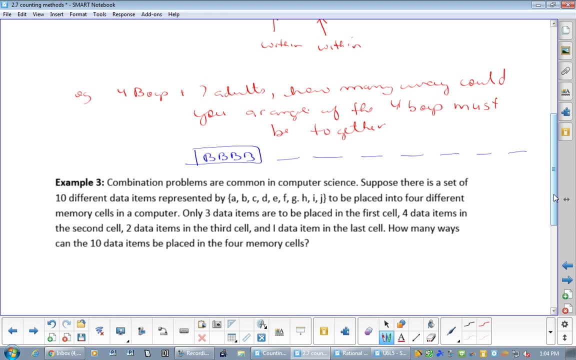 five, six, seven adults right now. do the adults have to stay together? doesn't say that, so the boys could go here, here, here, do you see that? so how many groups do we have or how many things do we have to do, have to be mixing around? no, these are. 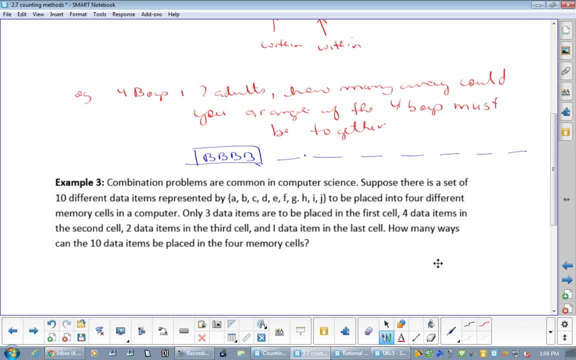 considered how many. this is one. so you do your eight factorial first. for the eight, see, we had seven adults and the one group- this is one group, isn't it? so it's considered like one thing. and then, how many ways can you do the four boys for factorial? so that's how you would. 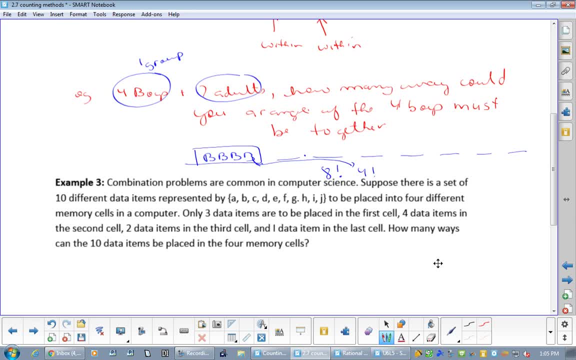 find the answer to that, because this is your seven adults here. it's times, okay, so this is the more common one that I've seen a lot. so you can arrange the four boys, but they stay together, how they can be arranged with the other things. and then, how many ways can you arrange the? 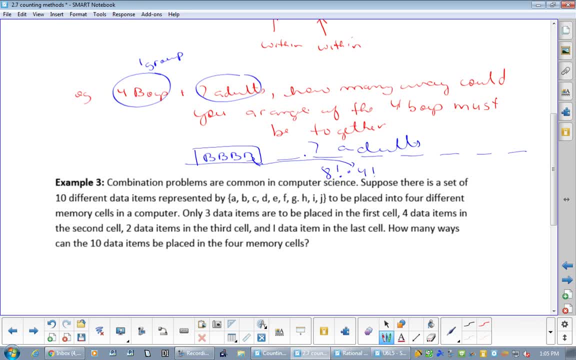 four boys, so it's number of groups, which is eight now one adults considered like a thing or a group. okay, so this is the four boys. so that's how you would do the four boys with seven adults. if the four boys must be together, how many different pictures could you take? and 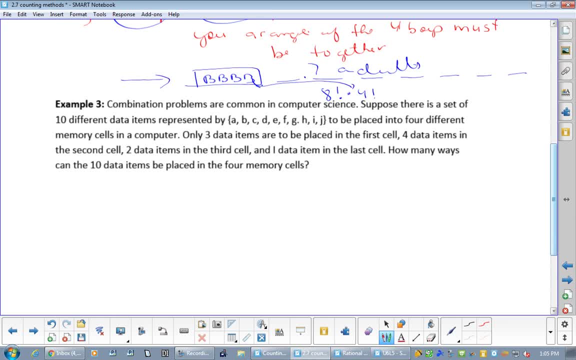 that this would definitely be a higher end question on the diploma, but I sure like when my students get those, as you can obviously imagine. okay, next one. now we're going to talk about the data items. so data items are common in computer science. suppose there's a set. 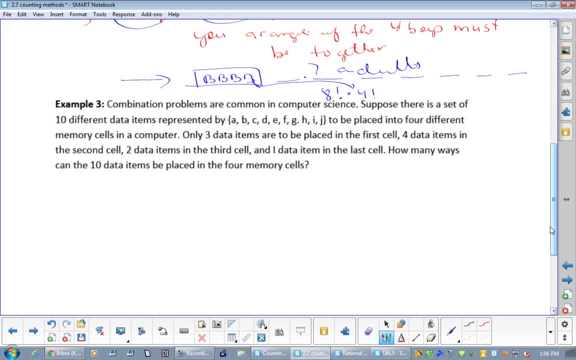 of ten different data items represented by ABCD of GL, the wage, to be placed into four different memory cells in a computer. only three data items are to be placed in the first cell for data items in the second cell, two data items in the third cell and one data item in the last. 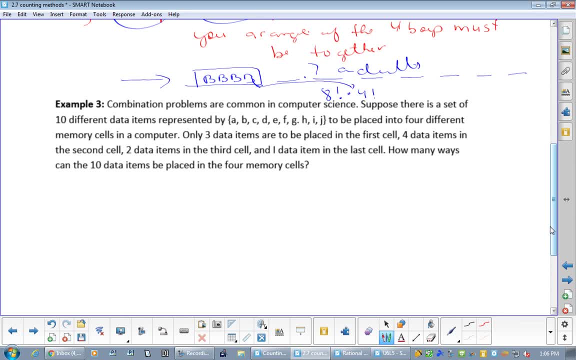 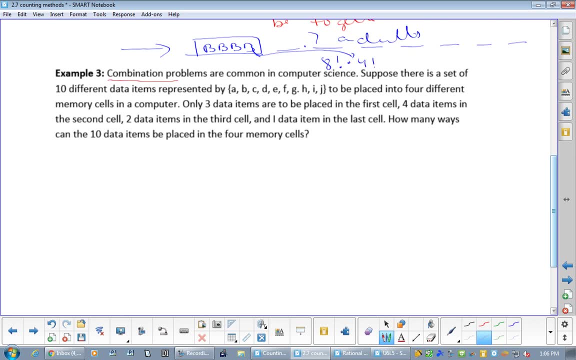 and the ten data items be placed in the four memory cells. now I'll admittedly this one. if they didn't start off with this, I would be assuming that you put memory in a different spot. it's going to like script your computer, right? but they said it's a combination, so okay, I'm good. 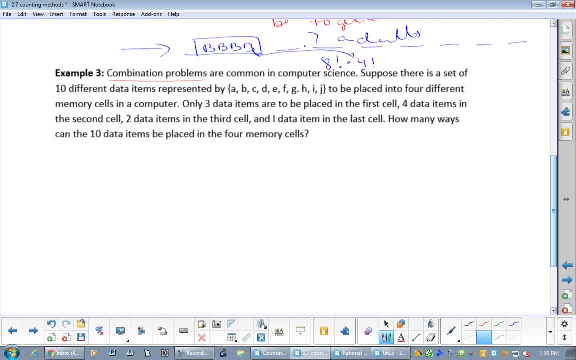 with that, I guess. so it says to be placed in four different memory cells: one, two, three, four. now, only three are to be placed in the first cell. so how many? how could I choose them? 10, choose three. so out of those 10, I guess they're. 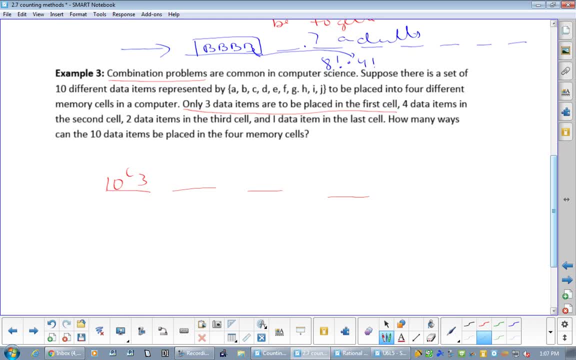 all identical, you know, but in that cell I'm going to put three of them, okay, so that's three items. in the next I have four items. the next one says two items and one item. okay, so how many ways now? and we're going to go because 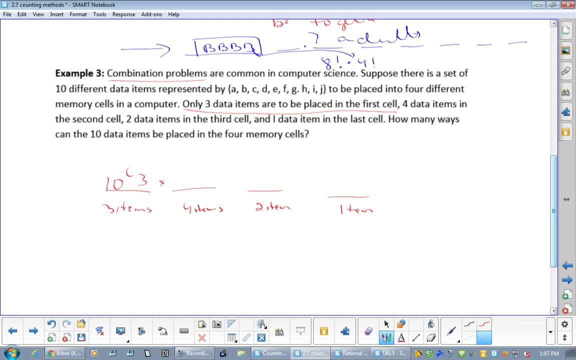 this is an or this is, and so I've three items in the first one and four items not, or four, because I got to use them all up, right? so now how do I choose the next four items? okay, that's awesome. see, I don't have 10 anymore, do I? because 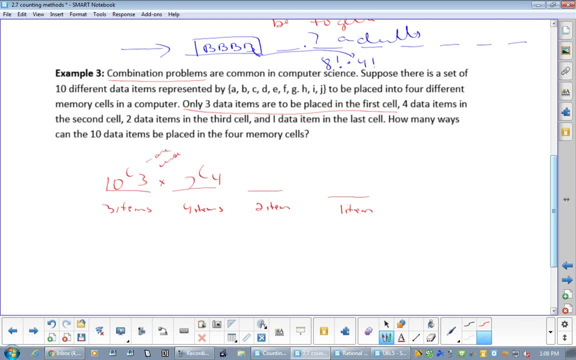 three are used. so I got 10, choose three, and now I have the seven left I could choose for those. how many different ways can they do that? okay, and now for the two items. I would have three, choose two and one, see one, and you would have to put those in your. 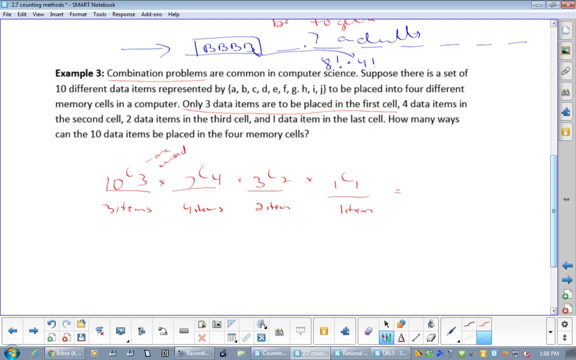 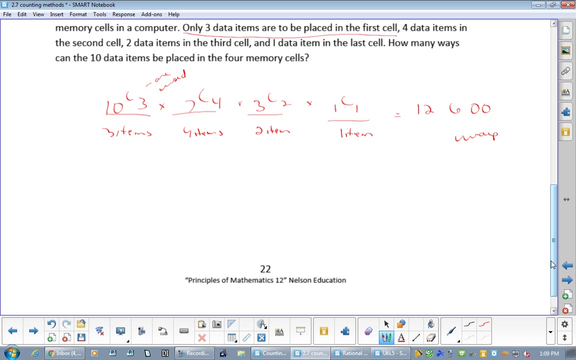 calculator. that's pretty arduous getting that in right. 10 math probability, see three times seven math probability, see right, you got to do all that and you'll get twelve thousand six hundred ways. okay, and I just want to an example for here how many. so this is a tricky one to. 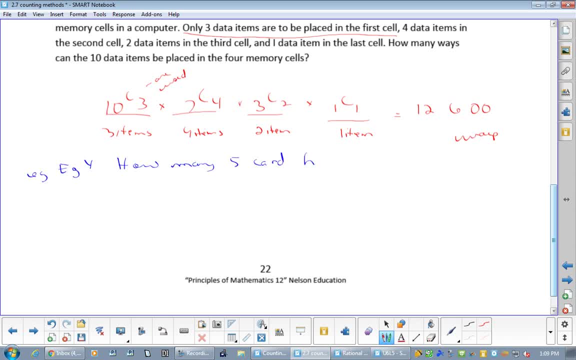 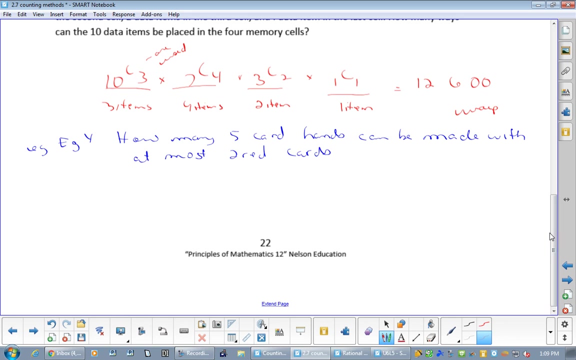 how many five card hands can be made with at most two red cards. we did at least yesterday. today we're doing at most can be at most okay. so who can tell me what this means? give me a hand. I would have at most two red cards, okay. so at most two red cards would be.